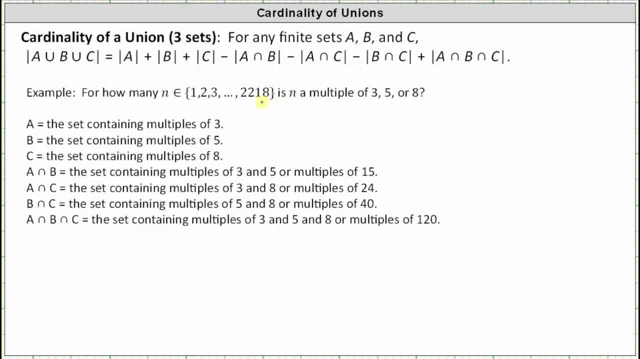 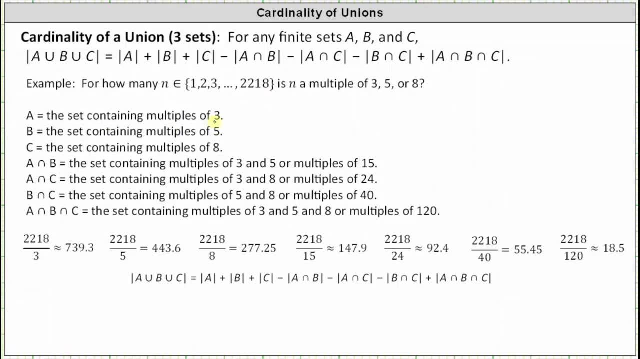 we can determine the cardinalities of the given sets using division. So, for example, for the cardinality of set A, which is a number of elements from the given set that are multiples of three, we take 2,218 and divide by three. 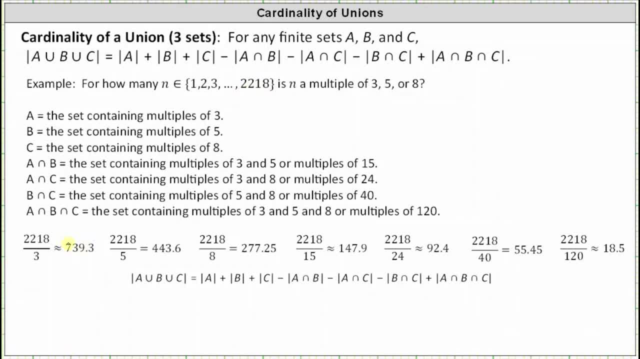 and whenever we get a decimal, we always round down regardless of the decimal. Notice how the quotient is approximately 739.3.. We round down to 739, which indicates the cardinality of set A equals 739.. There are 739 elements in the given set. 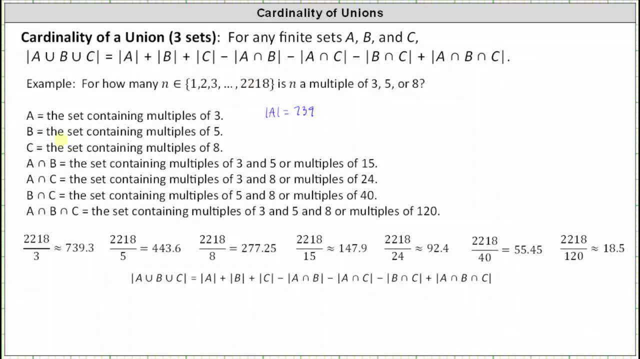 that are multiples of three. To determine the cardinality of set B, or the number of elements from the given set that are multiples of five, we divide by five and round down, which would give us 443.. The cardinality of set B is 443.. 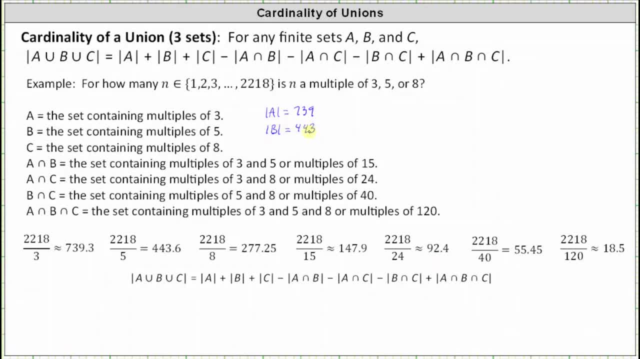 Let's line this up a little bit better. To determine the cardinality of C, which contains the multiples of eight, we divide 2,218 by eight and round down, which gives us 277.. The cardinality of set C is 277.. 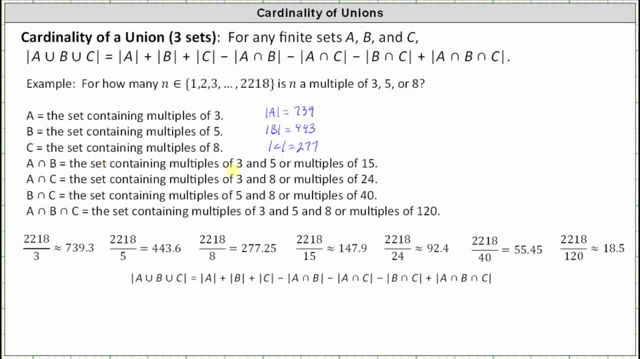 To determine the cardinality of A intersect B, which contains the multiples of three and five or multiples of 15, we divide by 15 and round down, which gives us 147.. The cardinality of A intersect B equals 147.. 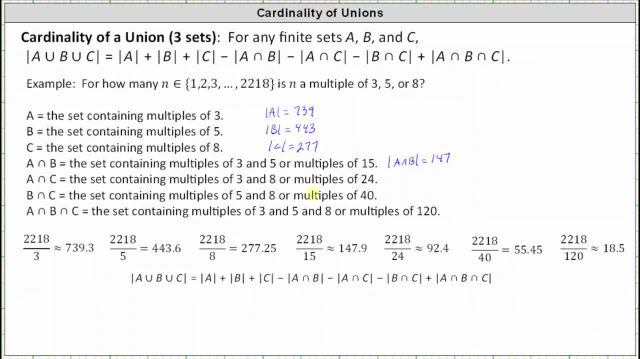 To determine the cardinality of A intersect C, which contains the multiples of 24,. we divide by 24 and round down to 92. The cardinality of A intersect C equals 92.. Next, to determine the cardinality of B intersect C. 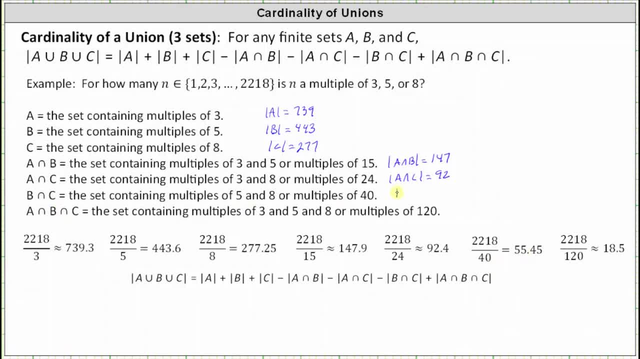 we divide by 40 and round down to 55.. The cardinality of B intersect C is 55.. And finally, to determine the cardinality of A intersect, B intersect C, which contains the multiples of three and five and eight, since three times five times eight is 120,. 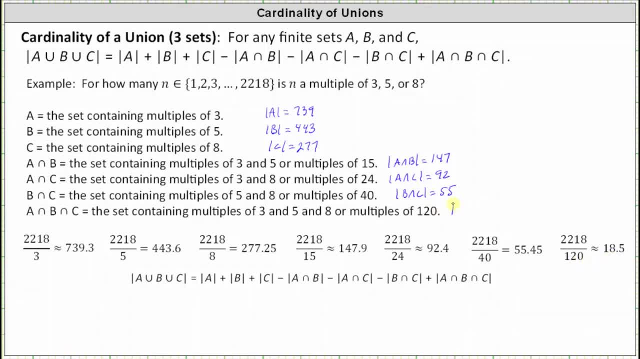 we divide by 120 and round down to 18.. The cardinality of A intersect B, intersect C is 18.. And now we have all the information we need to determine the cardinality of A union B, union C, which will give us a number of elements from the given set. 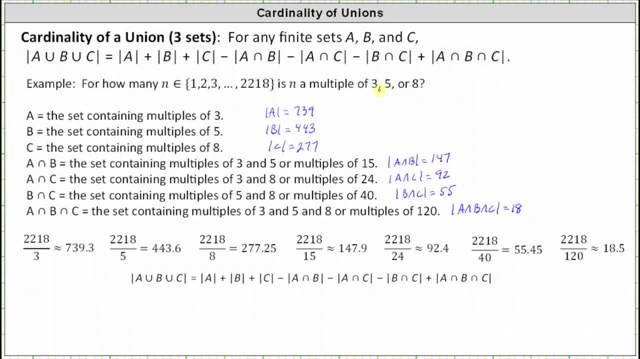 that are multiple, That are multiples of three or five or eight. Subbing in the cardinalities that we just found, the cardinality of A is 739, plus the cardinality of B, which is 443,, plus the cardinality of C, which is 277,. 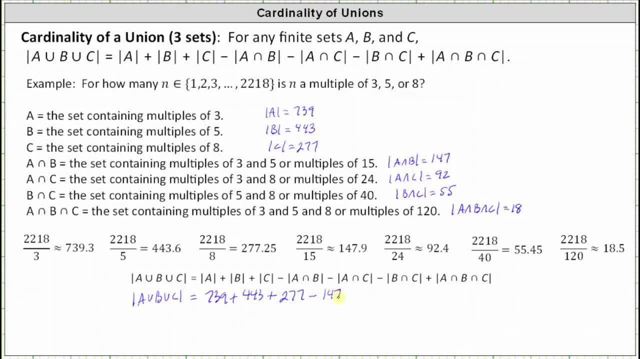 minus the cardinality of A intersect B, which is 147,, minus the cardinality of A intersect C, which is 92,, minus the cardinality of B intersect C, which is 55,, and then plus the cardinality of A intersect B intersect C. 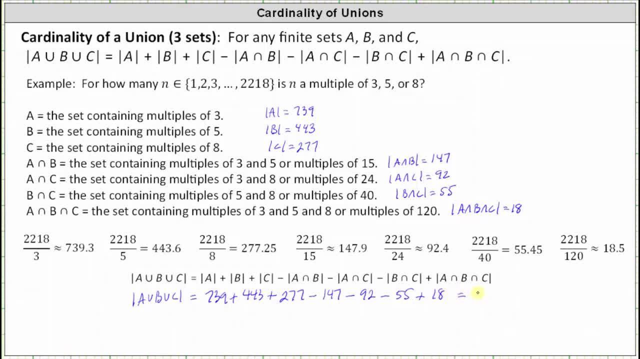 which is 18.. All this simplifies to 1,183.. So now we know the given set contains 1,183 elements that are multiples of three or five or eight. I hope you found this helpful. 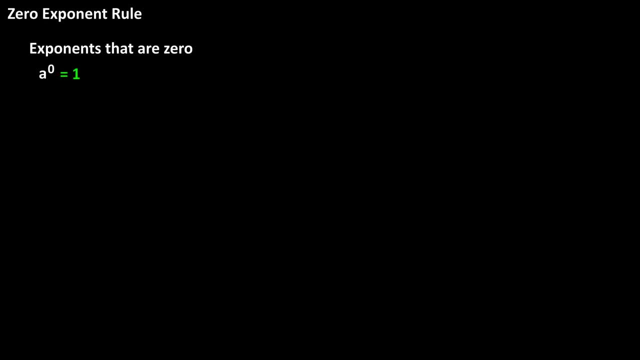 A number raised to zero, such as a raised to the zero, is equal to 1.. For instance, 3 raised to the zero equals 1, and we can use a quotient rule to show this As an example: 4 raised to the 4, divided by 4 raised to the 4.. The quotient rule tells us to subtract the bottom exponent from the top exponent. 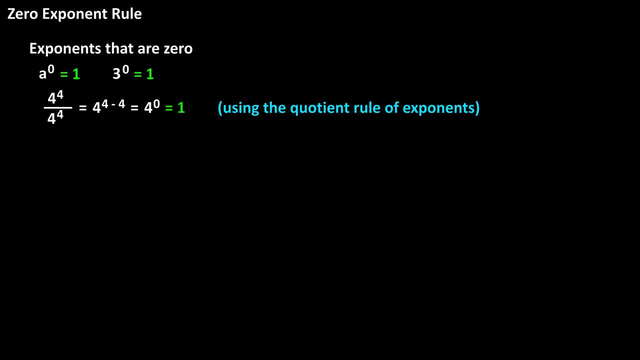 4 minus 4 is zero and we have 4 to the zero as our answer, which is equal to 1.. If we write this out, we have 4 times 4 times 4 times 4 as the numerator and 4 times 4 times 4 times 4 as the denominator. 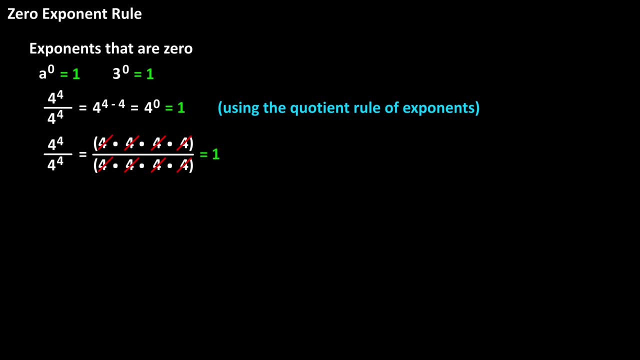 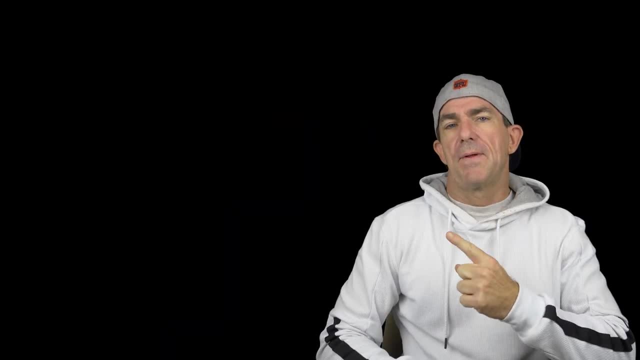 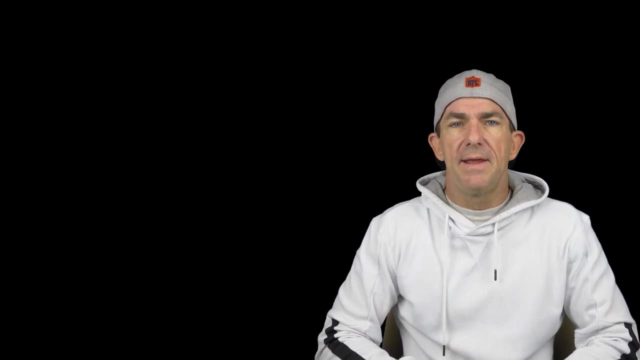 All of these 4's will cancel out and we have 1 as the final answer. same as before. Alright, my friends, hopefully you got something out of this video. I do have more videos right there for you Till next time I am outta here.